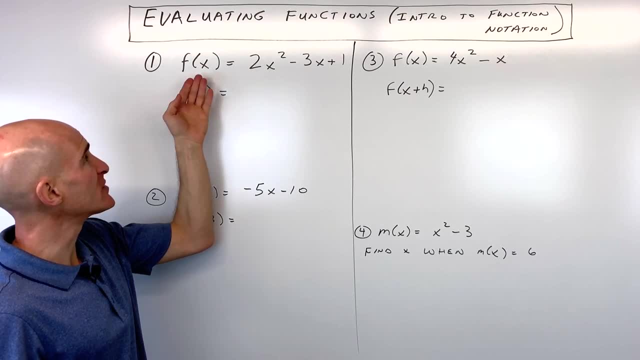 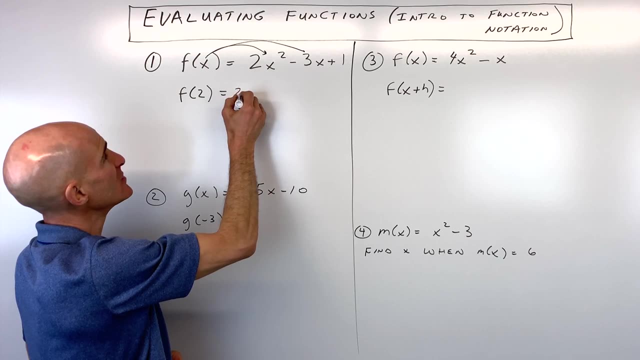 So if we wanted to evaluate f of 2 for this function, that just means that whatever is in the parentheses is going to go in place of x on the right side. So you can see this is going to be 2, and we're going to put 2 in place of x. we're going to square it minus 3 times 2 plus 1.. 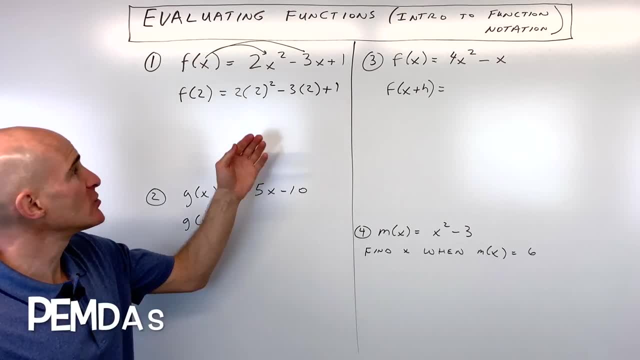 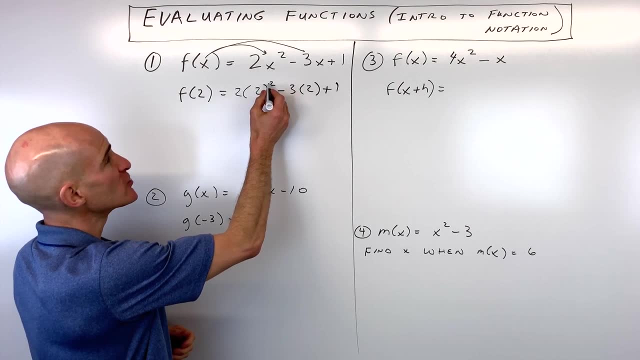 So the main thing here is to be careful with the order of operations You want to do the PEMDAS, the parentheses first, exponents, multiplication, division and then addition, subtraction last. So we've got: 2 squared is 4, times 2 is 8, minus 3. times 2 is 6, plus 1.. 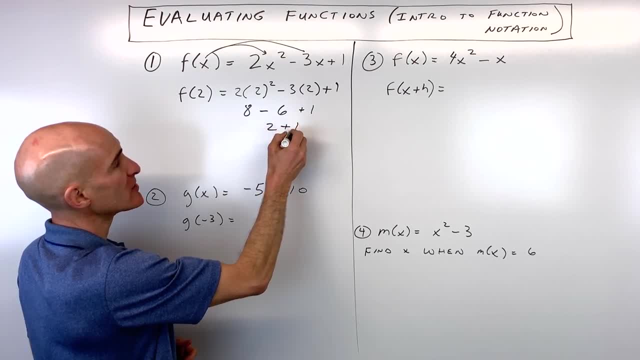 That comes out to 8 minus 6, is 2 plus 1, which is 3.. So we have f of 2.. f of 2 is equal to 3.. So 2 is our input, 3 is our output, and you've got it. 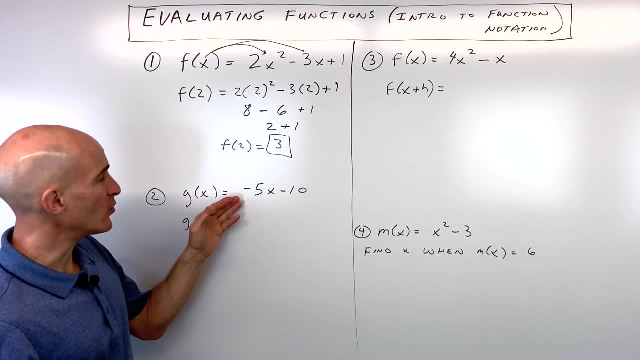 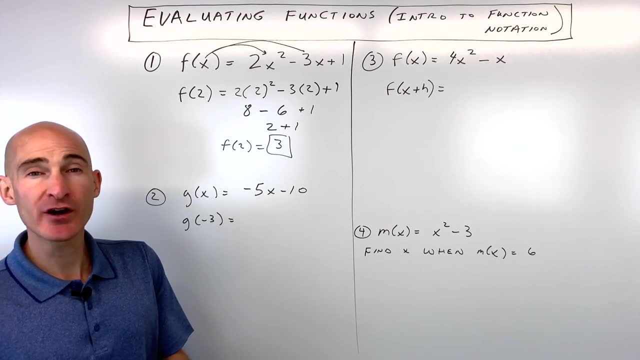 So let's go to another example, number 2. here We've got g of x equals negative 5x minus 10.. We want to find out what g of negative 3 is. Now, when you're using functions, you want to be really careful that you put your quantity, your substituting, in parentheses. 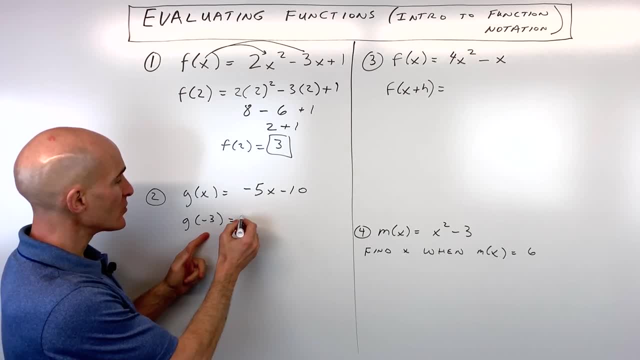 You want to treat it as a group, So that's an important concept. So here we've got negative 5, and then, in place of x, we're going to replace x with negative 3, and that's it. So all we have to do is do that. 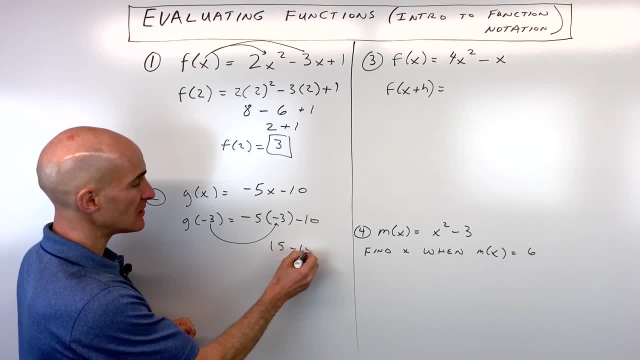 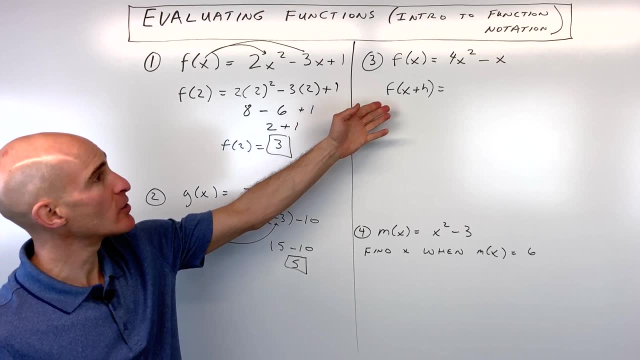 All we have to do is simplify Negative 5 times negative. 3 is positive 15, minus 10, which comes out to 5, and you've got it. So let's go to example 3, a little bit more challenging here. 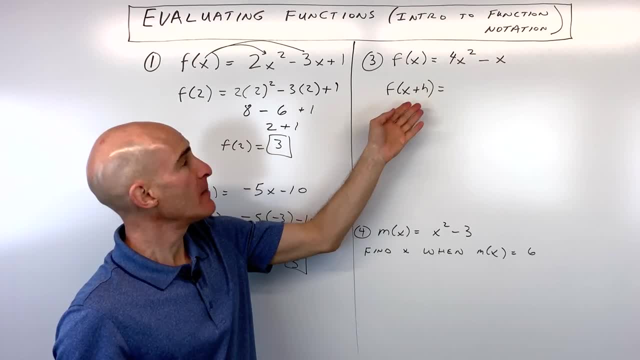 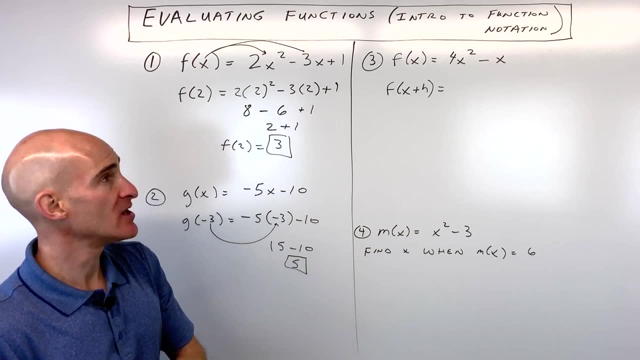 We've got f of x equals 4x squared minus x, and we've got f of x plus h. So we want to evaluate, when x is actually x plus h, the quantity x plus h. So same concept- Whatever's here in parentheses, goes in for x on the right side of the equation. 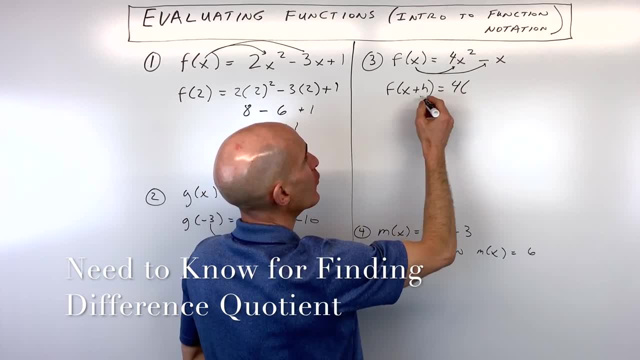 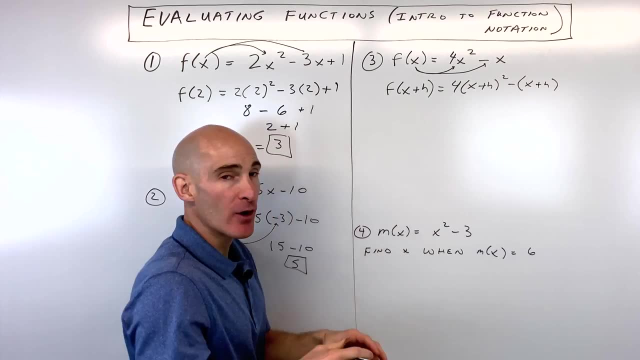 And again, you can have more than one x. So we've got 4x, We've got 4, and we're replacing x with x plus h, the quantity squared minus x plus h. Notice that I'm putting that quantity in parentheses, treating it as a group. 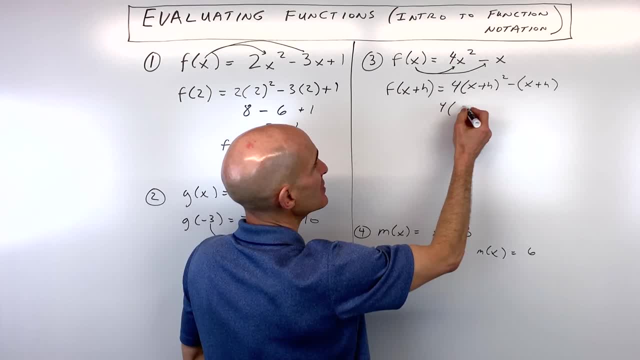 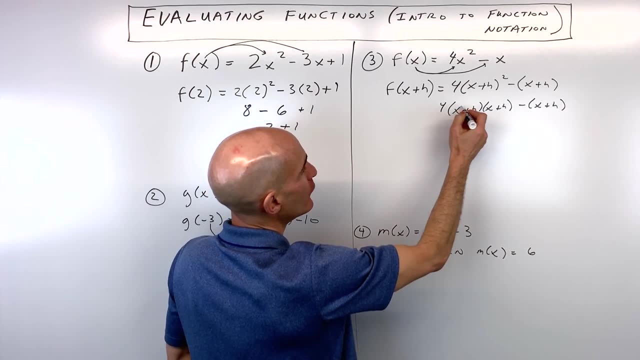 Now we just have to go back and simplify: x plus h squared is really like x plus h twice. okay, because you're squaring, You've got two of those And if you FOIL or do the distributive property, you get x squared plus x times h.